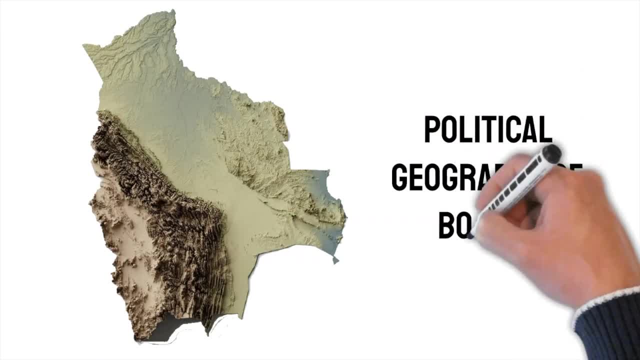 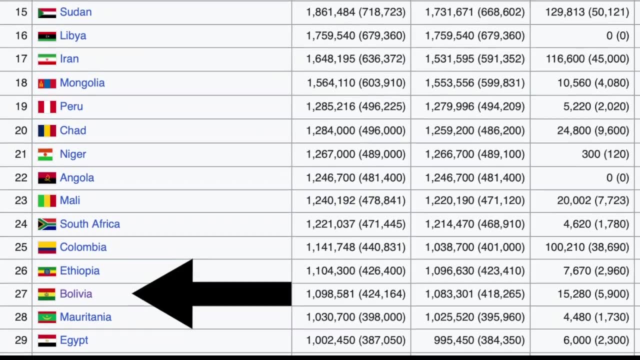 in such rugged terrain To see why. join me for this brief look at Bolivia's political geography. Bolivia is the 27th largest country in the world, with a land area of over a million kilometers, Once much larger. it is the second country in South America, other than Ecuador, to have lost 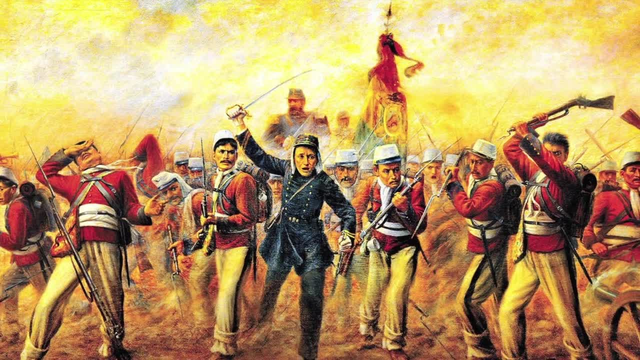 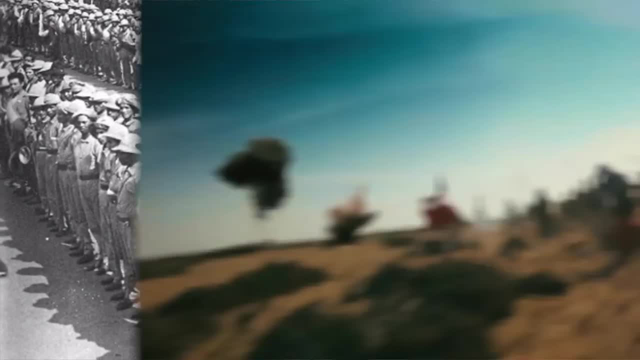 territory to every single one of its neighbors: Two were as a direct result of wars with Chile and Paraguay, and the others because of internal weakness compared to the neighboring countries. The one that stings the most, however, and is still a topic that pops up regularly in Bolivian 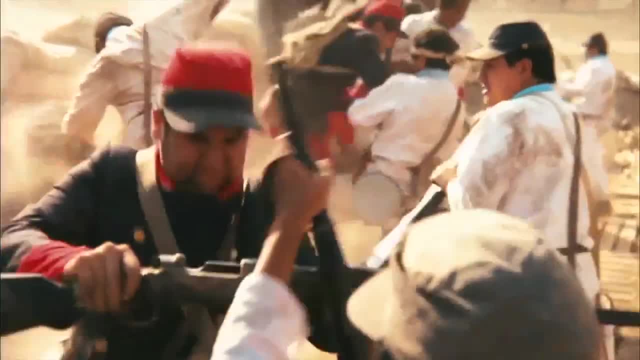 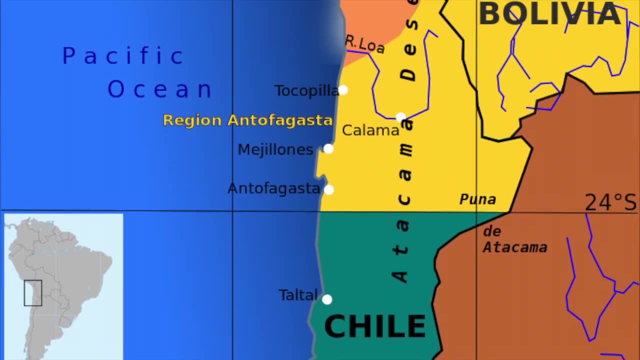 politics is the loss of the Atacama Desert to the Chileans in 1883 as a result of the War of the Pacific. The defeat gets regularly blamed for the present Bolivian underdevelopment because it made Bolivia a landlocked country And thus, ever since then, the Bolivians dream of. 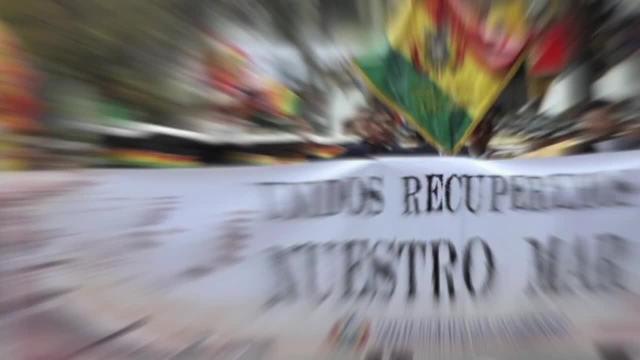 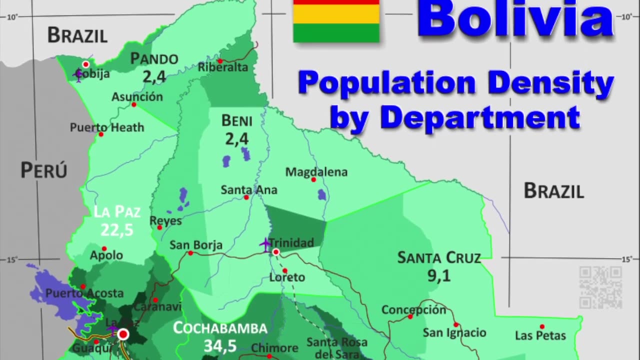 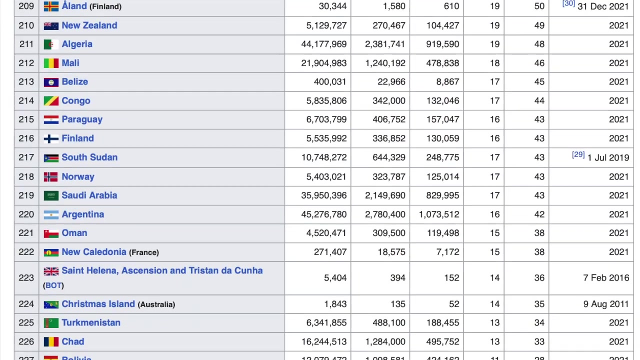 regaining their access to the sea. Meanwhile, if its size places it among the larger countries in the world, its population is much smaller, with the vast majority of its 12 million people living on its Andean side. In fact, the density of its population is so small that Bolivia's density 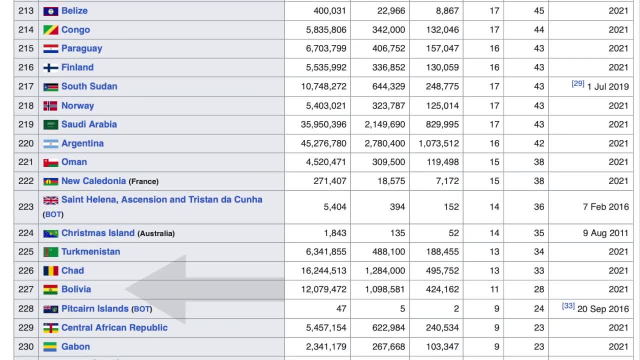 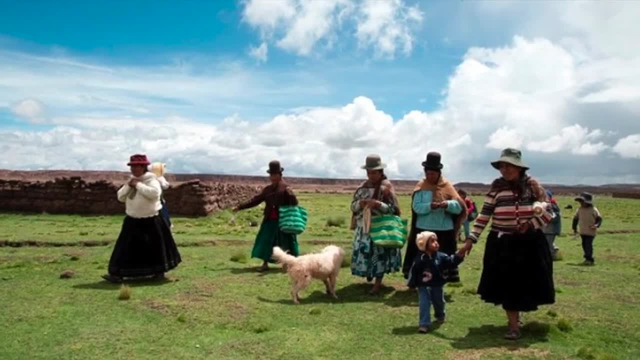 ranks as the lowest in Latin America and in South America, it's surpassed only by the Guayanes. Many of the Bolivian people who live on the Andean side of the Andean Sea in turn live in rural areas, making Bolivia one of the top five countries with the most rural. 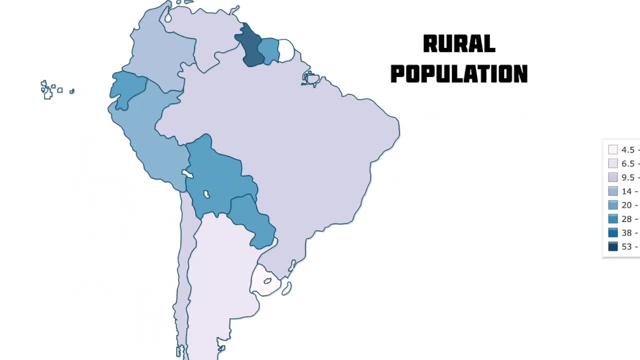 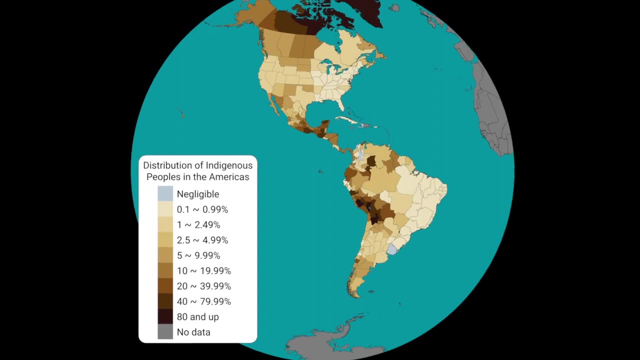 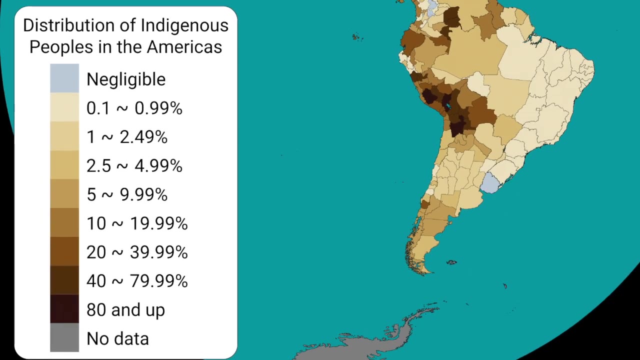 population in South America, just below Ecuador and Paraguay, with nearly 29% of its inhabitants living outside of cities. It is also the country with the highest proportion of indigenous people as a percentage of its total population, with nearly 50% self-identifying as such in the census. 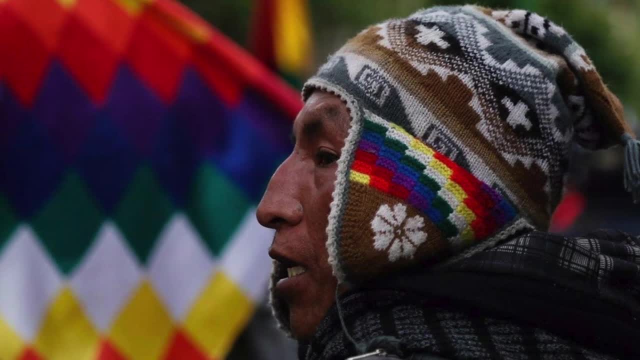 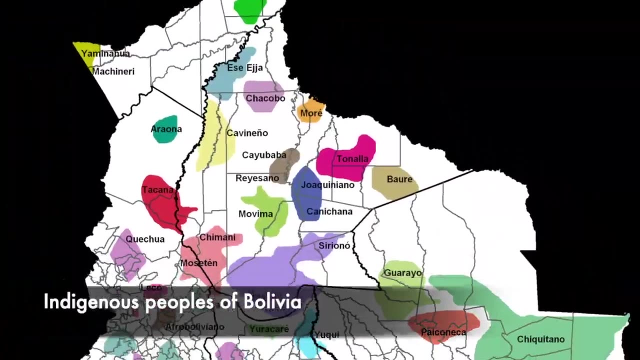 Although the image of indigenous people abroad is usually of those from the highlands, Quechua or Aymara speakers, Bolivia is the only country with the highest proportion of indigenous people in the Andes. In reality, the country has a wide array of native people all across the country who 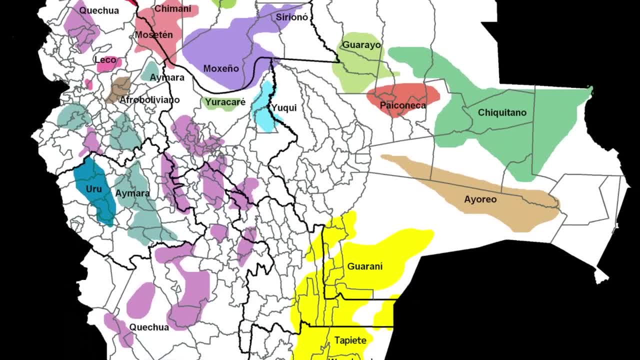 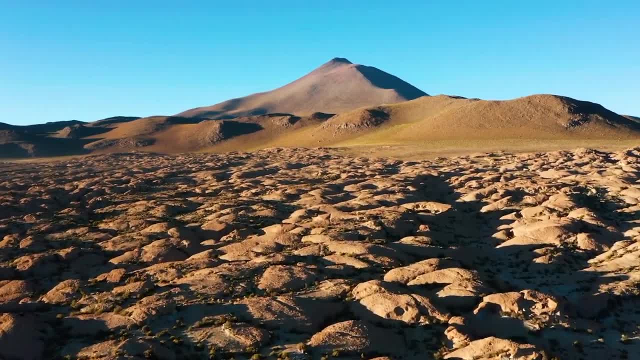 have little in common with those in the Andes. This is something that has been recognized in the country's official name, the Plurinational State of Bolivia. Bolivia's physical geography is dominated by the Andes, which frames its western side and shapes the rest of the country. This puts: 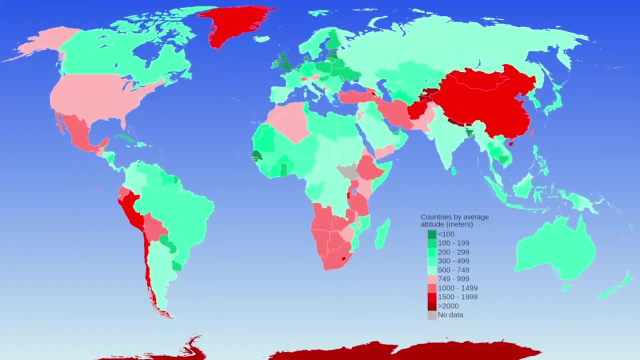 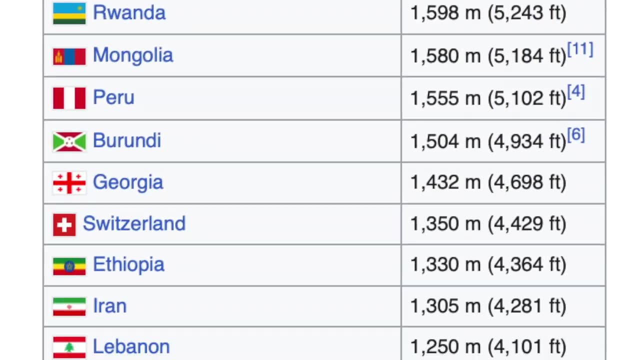 Bolivia among the top 25 countries with the highest elevation in the world, with an average height of 1,192 meters or 3,900 meters. Bolivia's national geography is dominated by the Andes, which is 911 feet, although it is still lower than both Chile and Peru, Because the Andes give 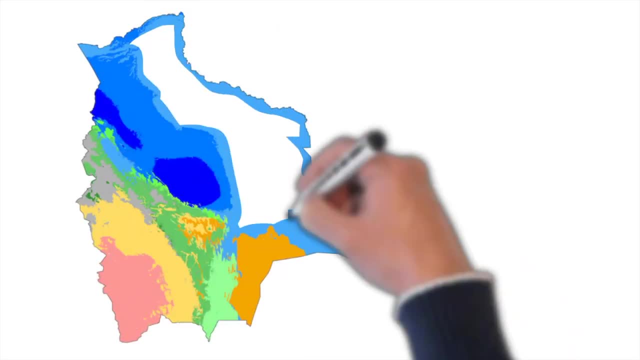 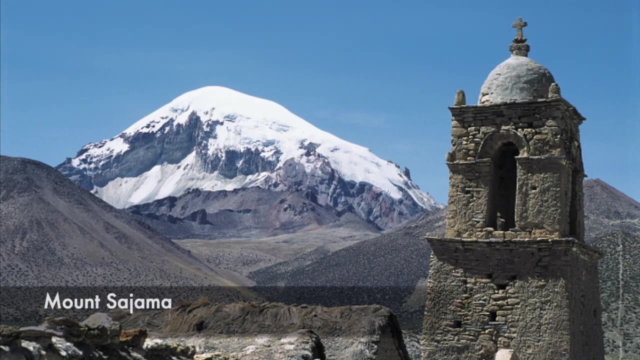 way to a tropical forest as one moves east. the country is home to a vast array of climates- a notable 14 in the Kopp and Geiger scale, ranging from polar frost in places like Mount Sahama, its highest peak, to various types of tropical forests on its eastern side, like the surrounding. 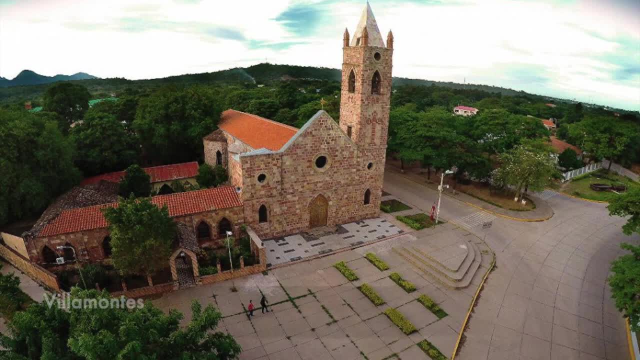 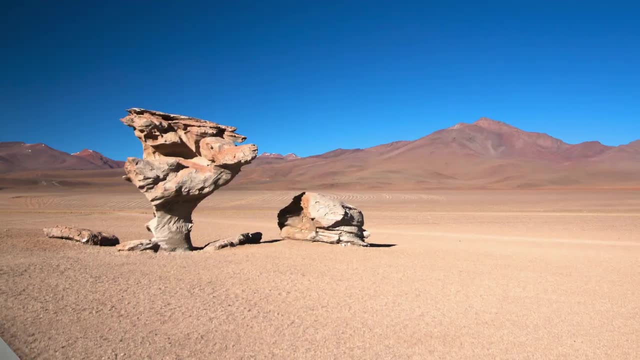 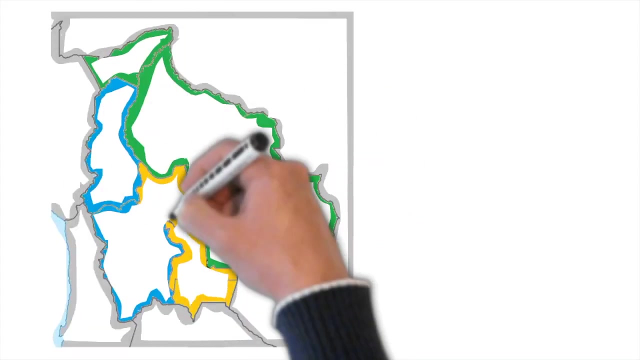 area near Villamontes, the hottest place in the country, with a low average temperature of 30°C or 86°F in August, and very arid places like the desert of Siloli on the border with Chile. Bolivians have traditionally collapsed the numerous ecological zones into three. 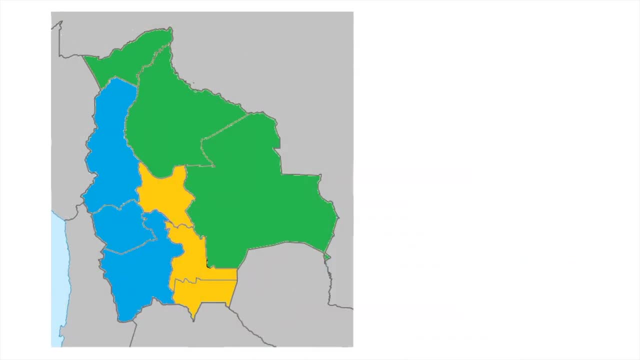 which coincide with the country's cultural regions. These are the Andean zone, usually called Altiplano, the sub-Andean central zone, generally called Valles, and the tropical lowlands, often called Llanos Orientales. The first and largest is the Llanos. 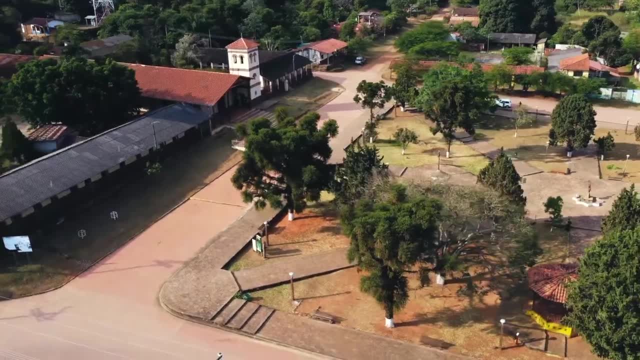 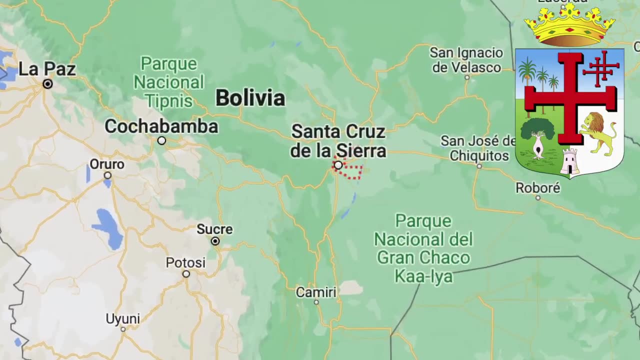 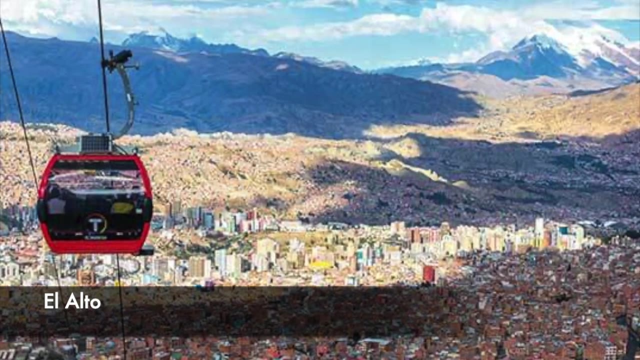 region, which encompasses 64% of the country's land area. It is also the least populated of the three, although the region's largest city, Santa Cruz de la Sierra, is also the biggest in the country, with roughly 2.4 million inhabitants, more than double El Alto, the next largest city. in Bolivia. Santa Cruz was founded in 1561 by Nuflo de Chávez as part of a colonization attempt from Spaniards based out of Asunción in Paraguay. For the Spanish, their expectations were not met. The town was too far from the 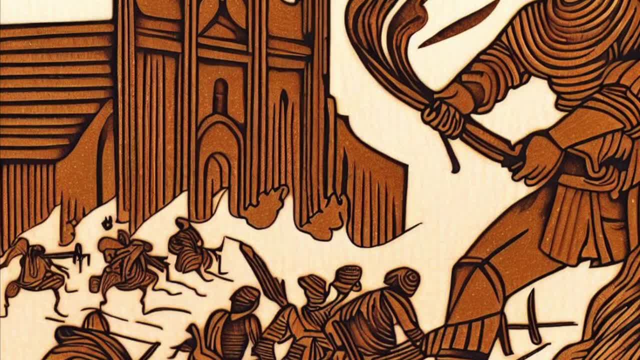 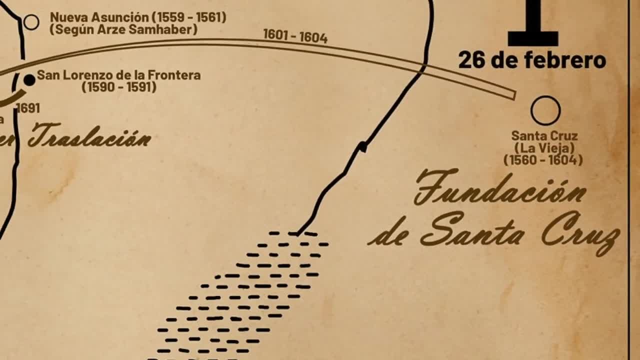 main markets, and Santa Cruz faced constant attacks from the local native peoples, including one that killed Nuflo himself in 1568, leading to the city being moved several times until its current location was finalized in 1621, leaving behind Santa Cruz la Vieja. 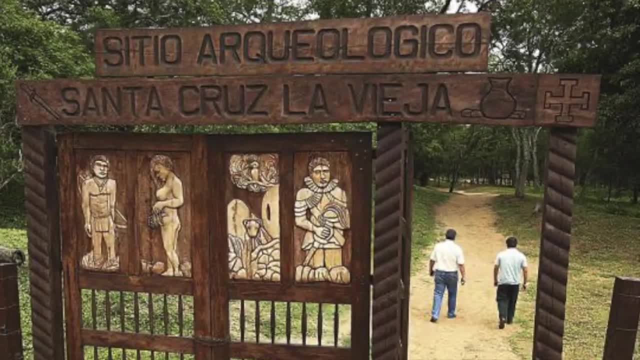 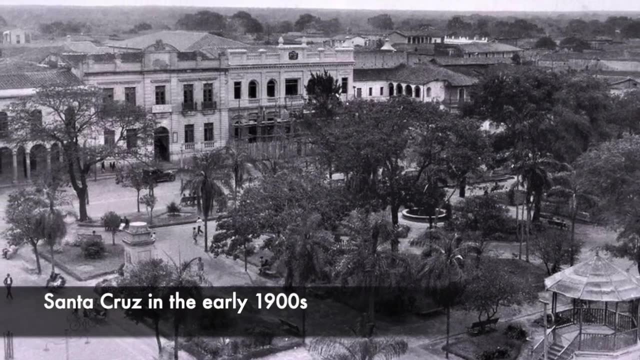 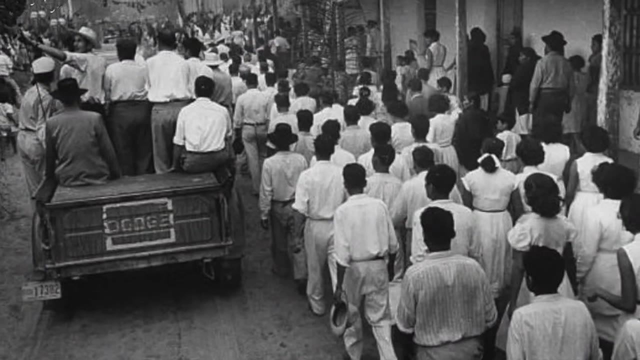 a little over 275 km to the east, ruins which you can still visit today. Over three centuries later, the city remained only a fraction larger than the original 10,000 people. What changed its trajectory was the construction of a highway in 1954 that connected Santa Cruz to western 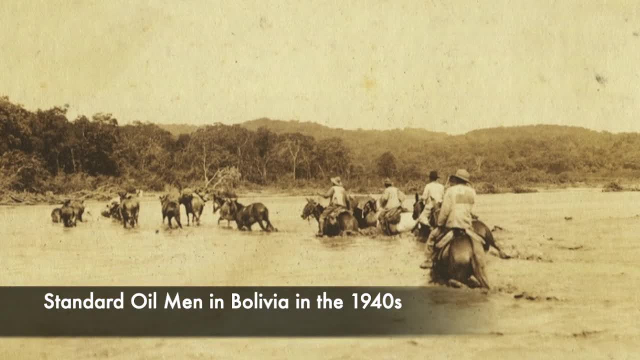 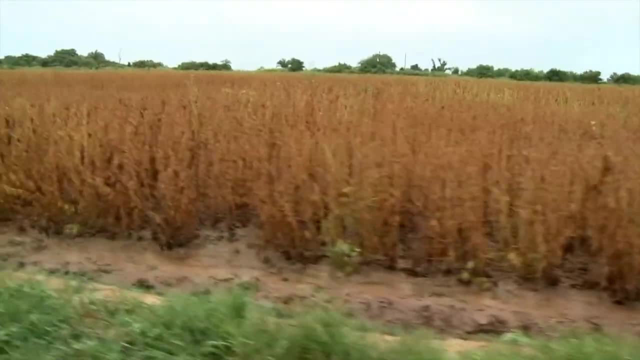 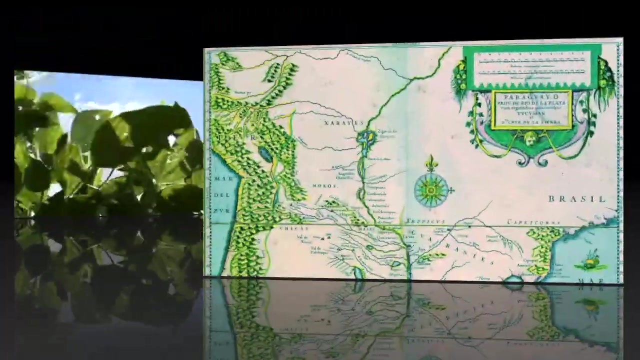 Bolivia's markets and the discovery of oil in the surrounding area. This turbocharged its economy, making it a center for hydrocarbons, but also an agricultural hub, as its hinterland became a breadbasket for the country, producing corn, rice and wheat. Historically, the rest of the 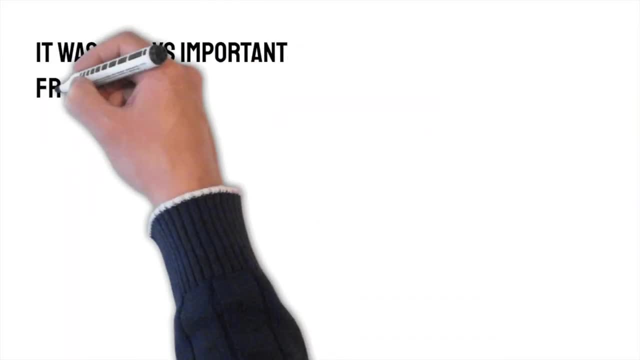 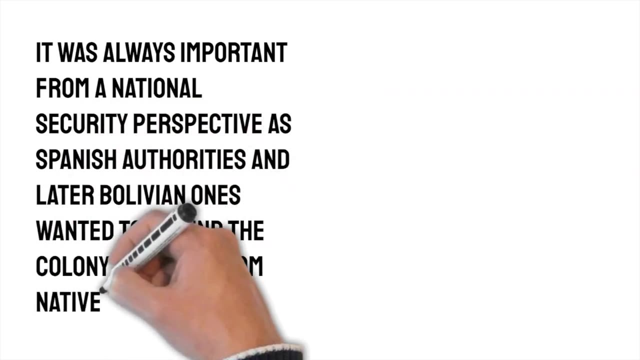 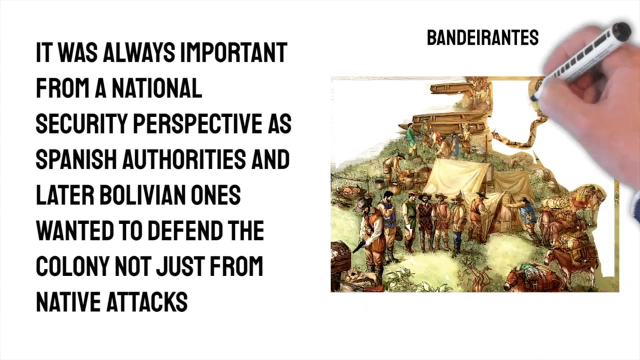 city was also quite isolated, although it was always important from a national security perspective, as Spanish authorities, and later Bolivian ones, wanted to defend the colony not just from native attacks but also encroachment from the Banderanches, Brazilian settlers, who did much to expand Portuguese territorial claims in the area, And so the Spanish Crown. 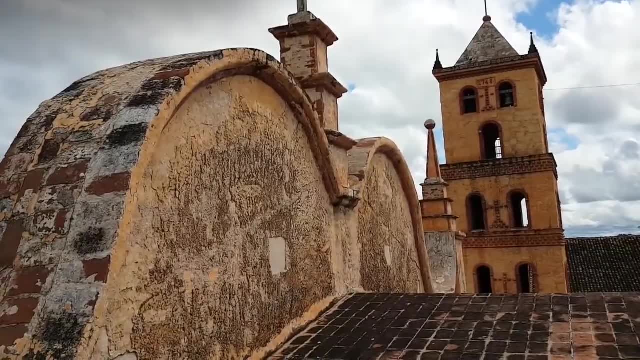 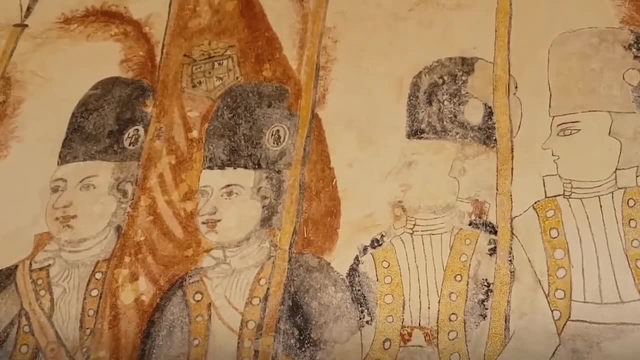 saw to the construction of Jesuit missions in the savannah near Santa Cruz, an area known as Chiquitania at the time, which aimed to convert the natives and establish Spanish authority. These missions have survived largely intact and have since been declared UNESCO heritage. 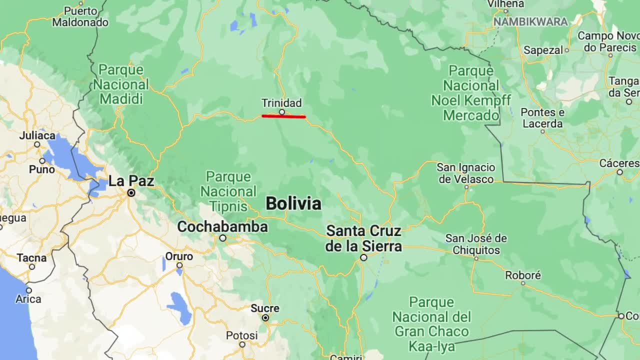 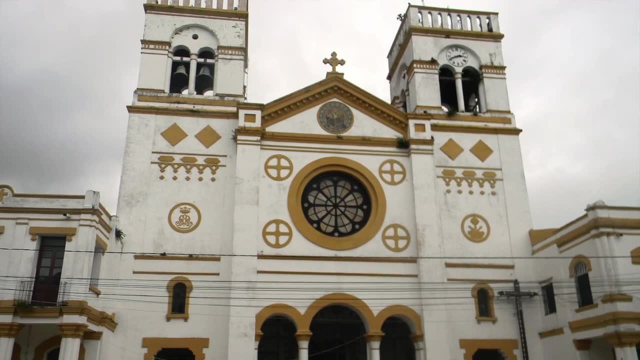 sites. Trinidad, a town in the northeastern part of the country, had a similar origin story and was founded around the same time, in 1686, but little of the original mission survives. Security considerations of this region continued after Bolivia became landlocked. 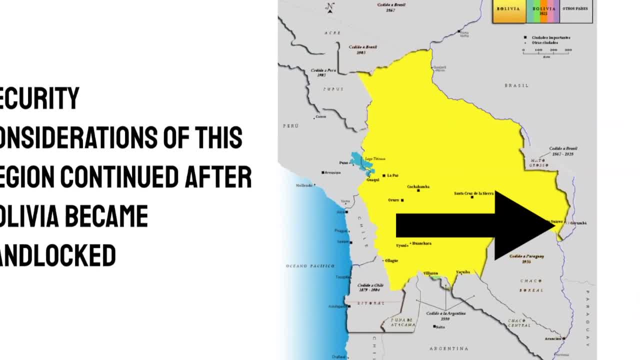 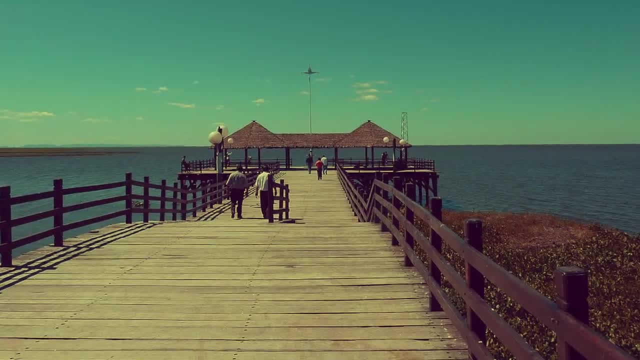 as national authorities sought a way to have access to the Atlantic through the Paraná River. In 1875, a town named Puerto Suarez was established where the river reached Bolivian territory. It worked as such until the 1940s, when sedimentation 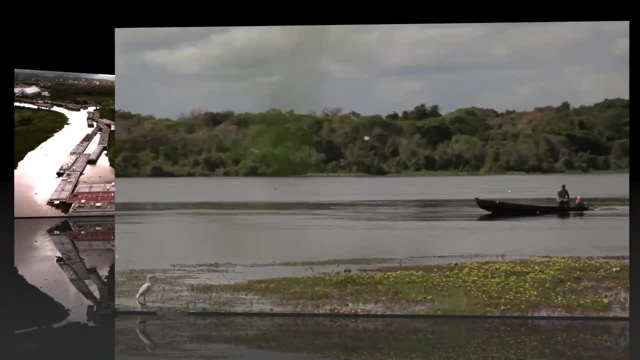 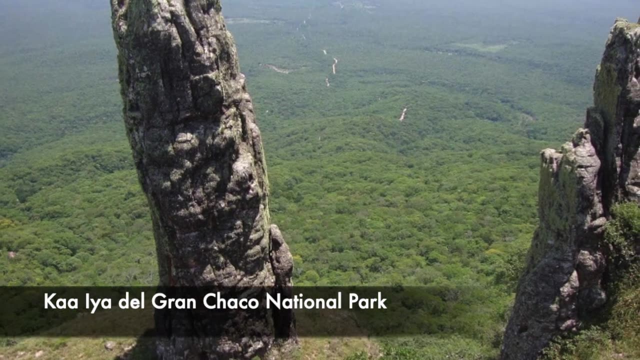 in the nearby lake prevented larger ships from reaching it. The Llanos region also comprises some of the most important national parks in the country, including the largest one in Bolivia, the Caia del Gran Chaco, which has a size larger than Belgium and happens to be the largest wooded. 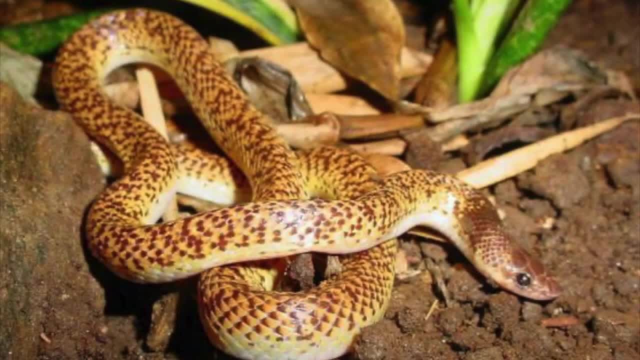 tropical area in the world. It features a number of snakes and mammals, like the pampa snake, guanacos chacoan mara and conovera, which are also known as guanacos chacoan mara. 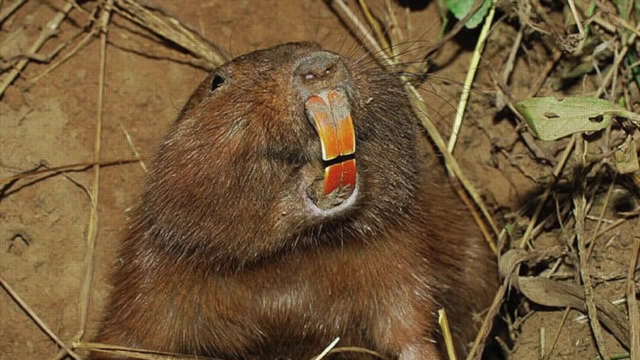 and conovera, which are also known as guanacos, chacoan mara and conovera, which are also known as tucotuco, as well as a number of endangered species like the tagua. The popularity of the 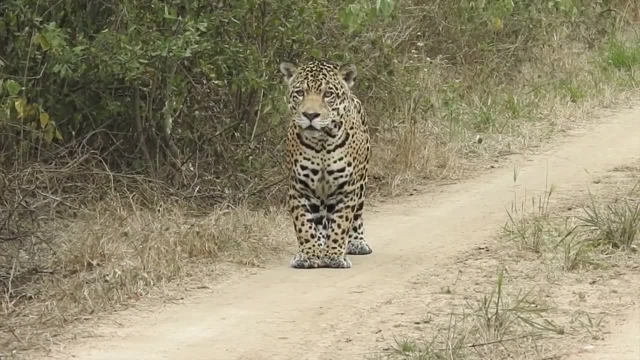 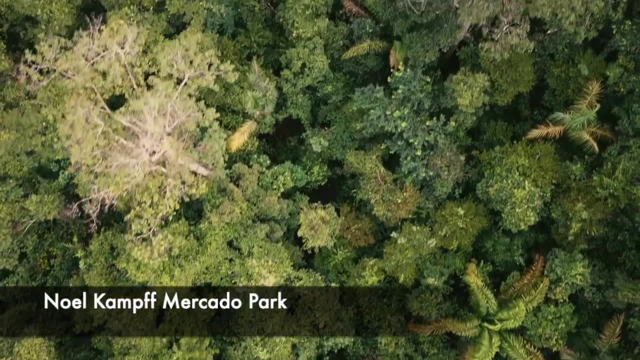 park, however, stems largely from the fact that, if you visit, there's a high likelihood you'll see a jaguar or some other big cat in its natural habitat. There's also the Noel Kempf Mercado Park on the border with Brazil, featuring an iconic waterfall, an untold number of mammals and 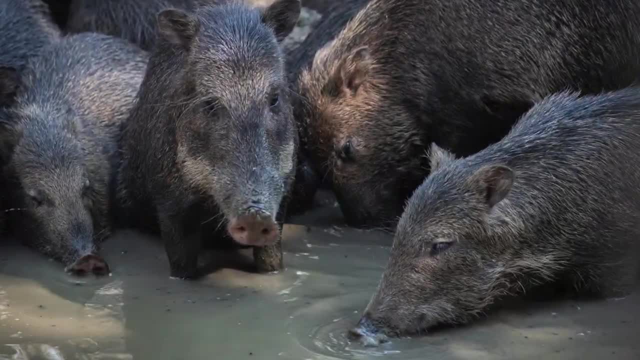 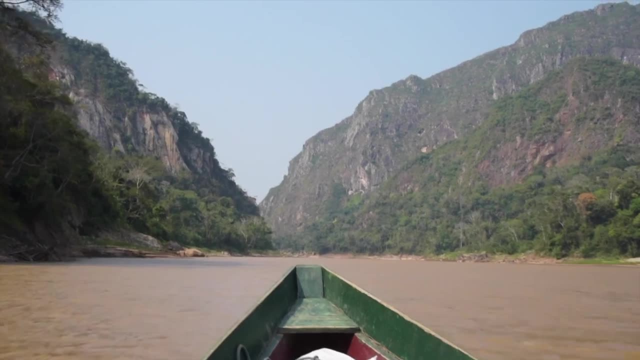 reptiles, including the chancho de tropa and borochi. Finally, there's Madidi National Park, which is not just one of the most biologically diverse areas in the country but the planet, as it includes an incredible range of ecosystems from high-altitude. 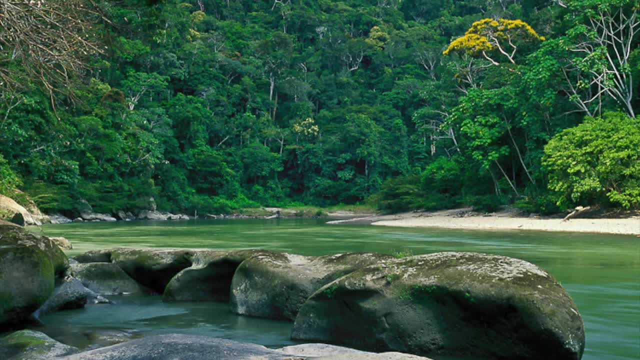 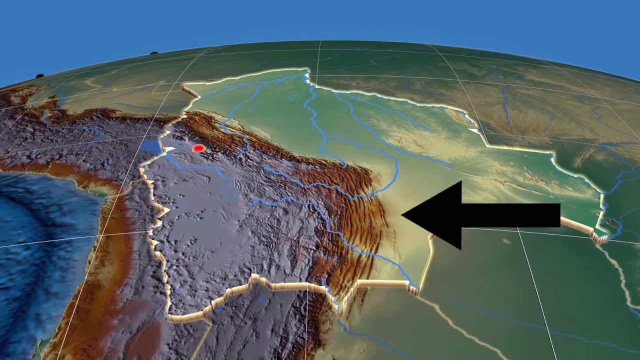 grasslands to cloud forests, lowland tropical forests to pristine lowland savannas. It was also here, at the edge between the Llanos and the Valles zone, that the event to have happened on Bolivian soil most likely to be known by foreigners, occurred. 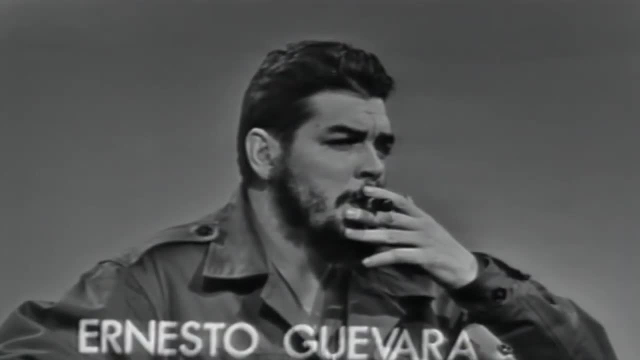 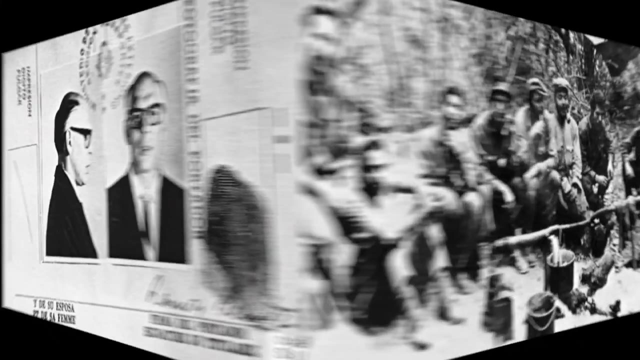 the capture and execution of Che Guevara. The Cuban revolutionary had entered Bolivia in November 1966 with the intention of bringing revolution to the country, but had little success and was instead captured by the Bolivian army on October 8, 1967.. He was 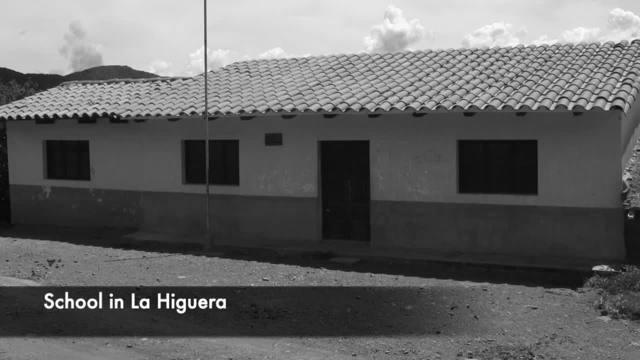 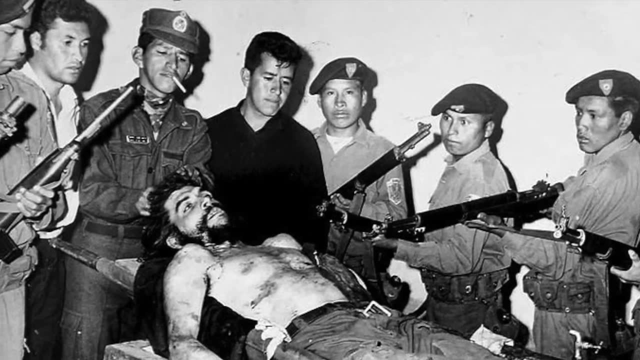 then brought to a nearby schoolhouse in the hamlet of La Higuera, where he was detained until his execution the next day in the afternoon. Afterwards, his body was taken to Valle Grande, a town about two hours away, where his body was pictured to document his death. 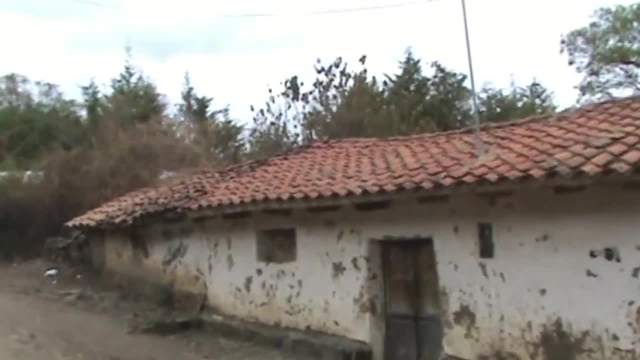 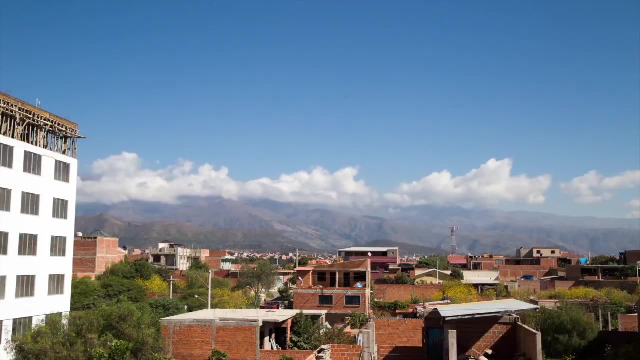 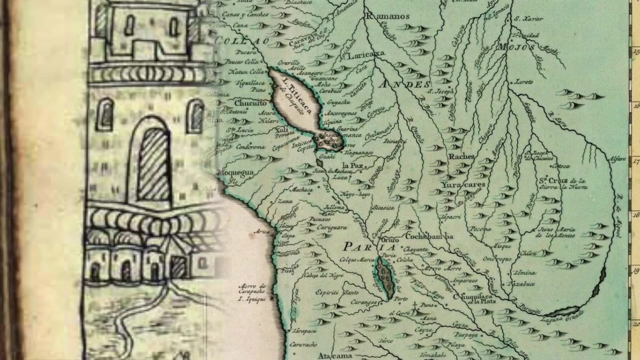 Since then, chess fans have been retracing his steps. The second zone is the Valles region, the smallest of the three and the least populated, with slightly less than a third of Bolivian people living there. The area was the center of Spanish power and learning during colonial times. 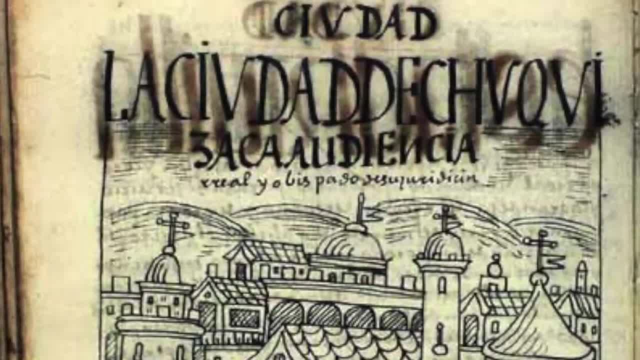 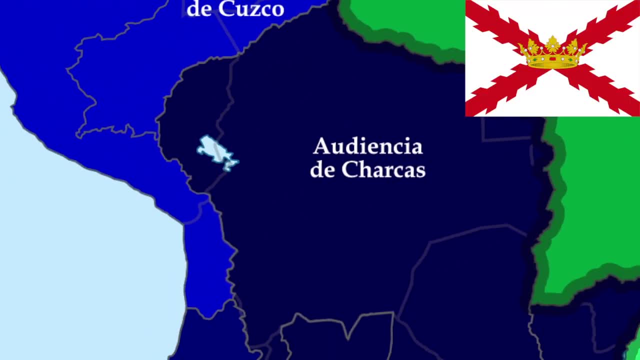 Its main city, Chuquisaca, later renamed Sucre, was founded in 1538, and a little over two decades later was made the seat of the Audiencia de Charcas, a judicial demarcation that, in practice, gave province-like autonomy to the region. 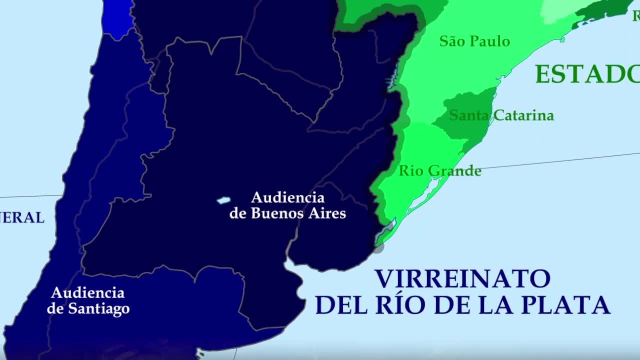 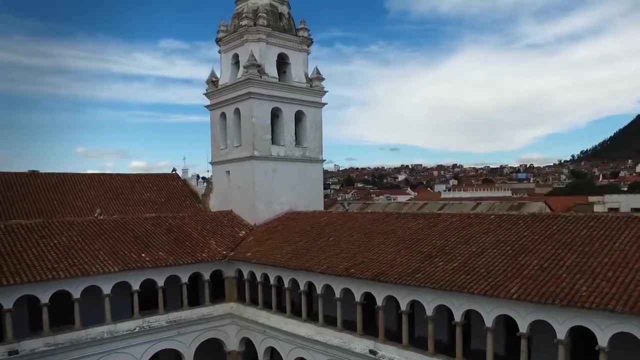 First within the Viceroyalty of Peru and later the Viceroyalty of La Plata. Its university, San Francisco Javier, was established in 1624 and was one of the most important in the western hemisphere at the time. 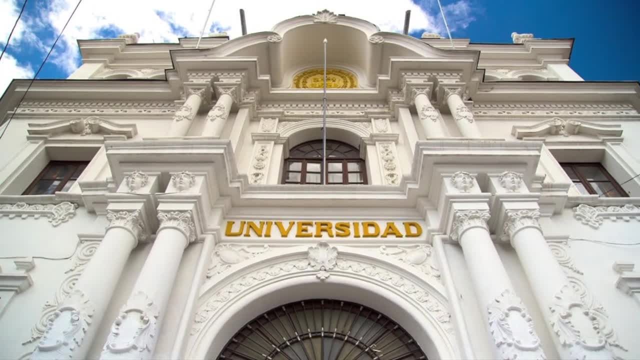 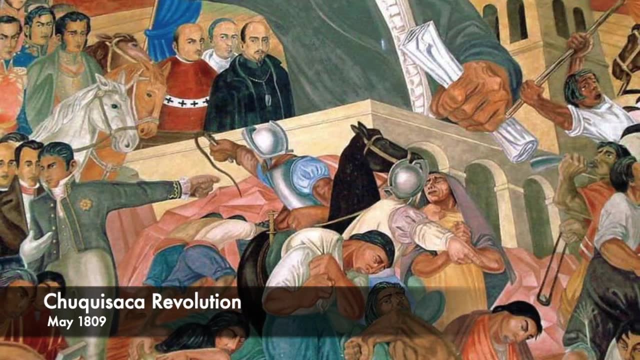 Because of its status. when Napoleon invaded Spain in 1808, appending Spanish authority in the Americas, the elites in the city were the first to call for independence. The Chuquisaca Revolution, as it came to be known, sparked similar movements elsewhere in Bolivia. 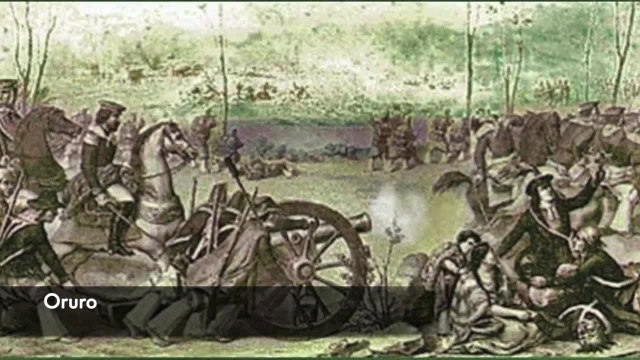 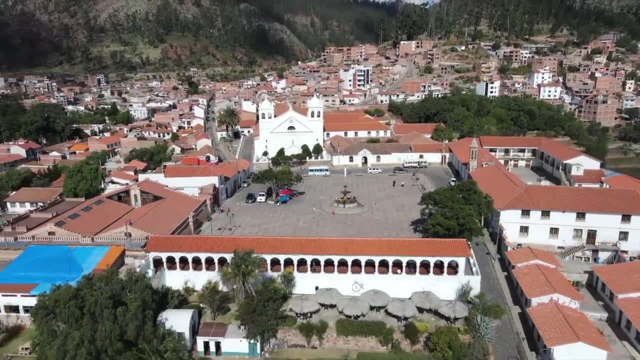 in La Paz, Cochabamba and Oruro, which would eventually lead to independence for the country. The longest Spanish presence left its mark everywhere in the city. You can see it not just in its architecture, which gained its status as a UNESCO World Heritage Site in 1991, but also 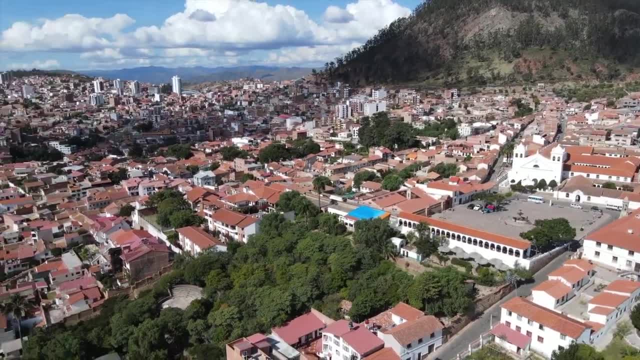 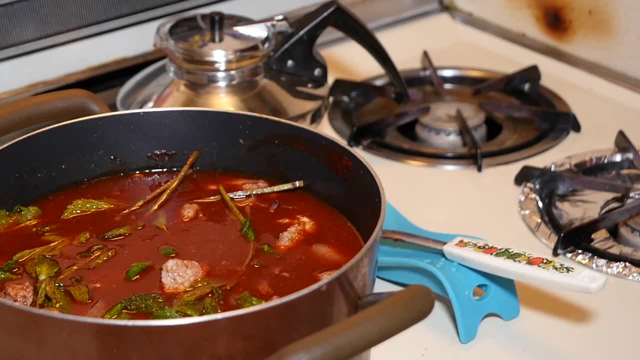 in the food. Two of the most traditional Chuquisaca dishes, for example, are made out of pork, a popular ingredient in Spanish cuisine that the Spaniards brought to the Americas. The first, fritanga, is fried pork with ají, a local Bolivian pepper, and the second are chorizos. sausage that today still marks for a very cheap lunch. The region's centrality in Bolivian history began to subside after independence, especially once the capital was moved to La Paz in 1898, but two important subsequent events should be noted. The first was that it was the birthplace. 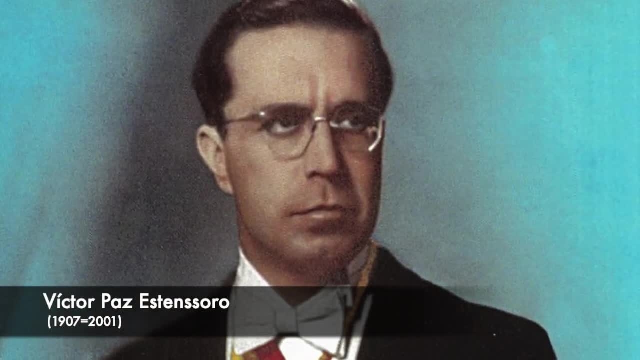 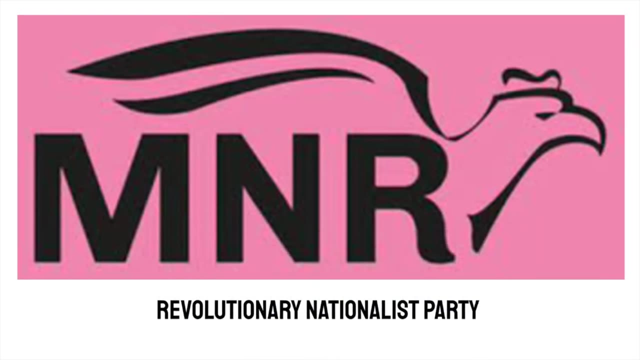 of Víctor Paz Estensoro, a man born in Tarija in 1907, who would go on to found the Bolivian Revolutionary Movement, or MNR, the most important Bolivian party of the 20th century. The other was: 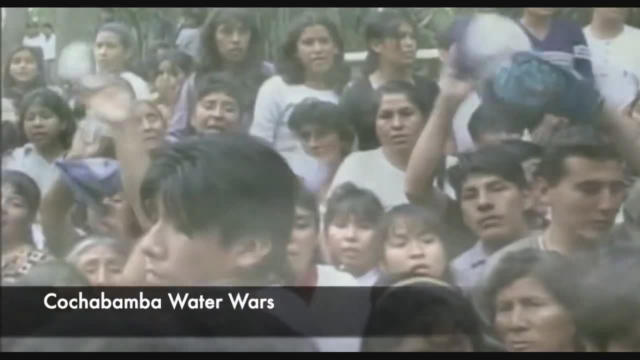 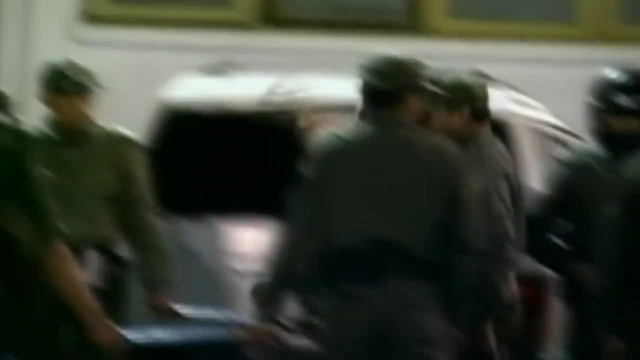 the Cochabamba Water Wars- The Bolivian Revolutionary Movement, or MNR, was founded in 1898, a series of popular revolts against the privatization of water in late 1999-early 2000, which would shape the conversation in Bolivian politics for the next two decades. 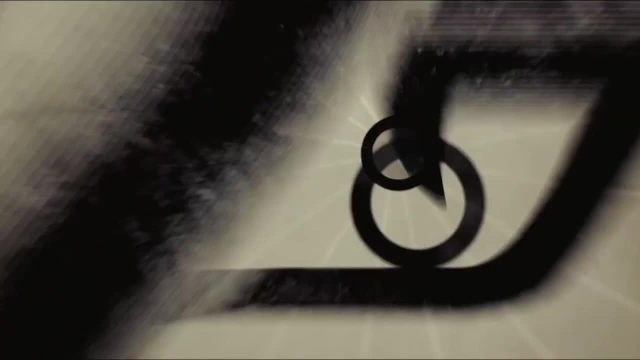 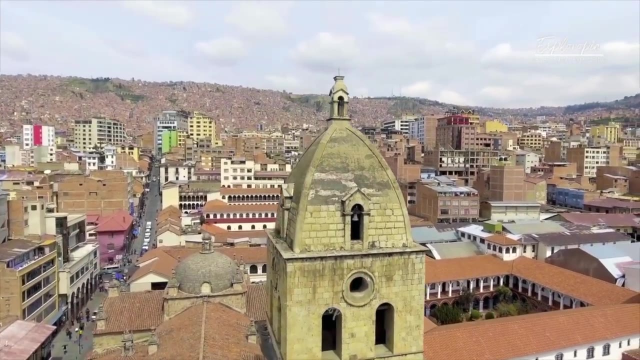 and would even inspire part of the plot of the James Bond movie Quantum of Solace. The final zone is the altiplano, the western part of the country, framed by the Andean mountain ranges. Historically, this zone was the home to some of the most studied ancient peoples. 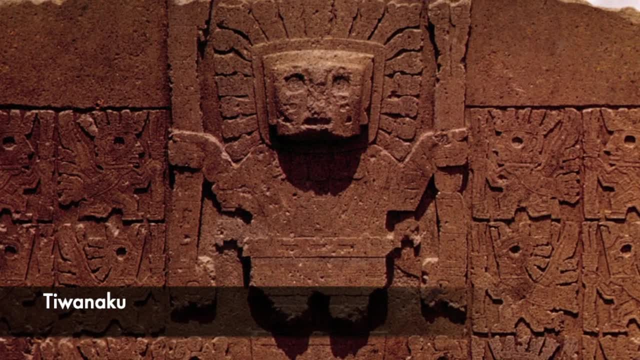 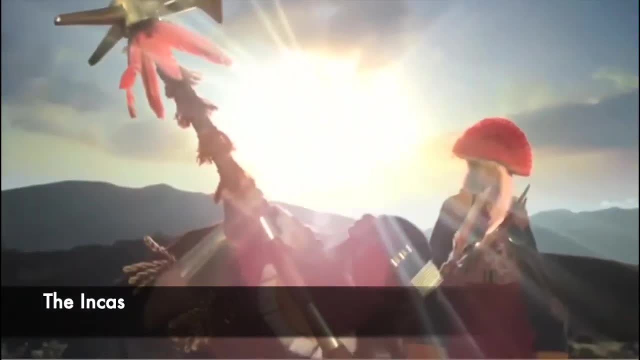 in the country. These include the Tiwanaku, a civilization that developed on the outskirts of Lake Titicaca, who would dominate the region for 400 years, and, of course, the Incas, who began conquering the region in 1438 and would eventually incorporate much of the altiplano into their empire as the Cuyasuyu province. The ruins of both dot the landscape, but the most important is the eponymous city of Tiwanaku and the Isla del Sol, or Island of the Sun, where the Incas believed the sun had its dwelling place. Their influence is still evident everywhere. 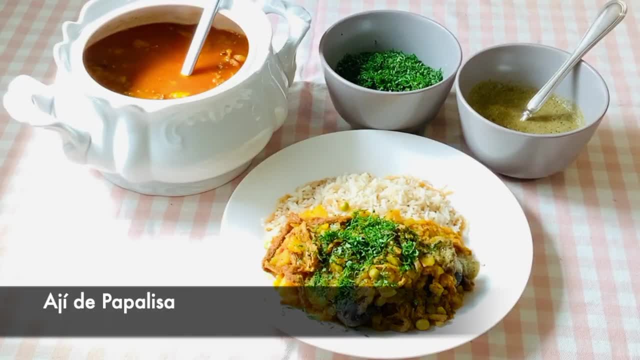 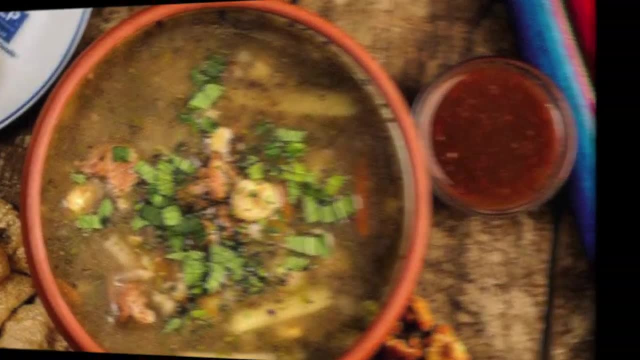 especially in the food, with typical dishes like ají de papaliza and chairo, both potato-based dishes, although the latter is a stew that also includes llama meat. Once the Spanish arrived, the altiplano gained not just national but global importance. That 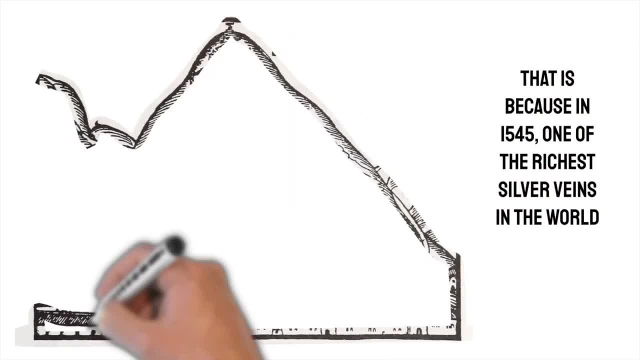 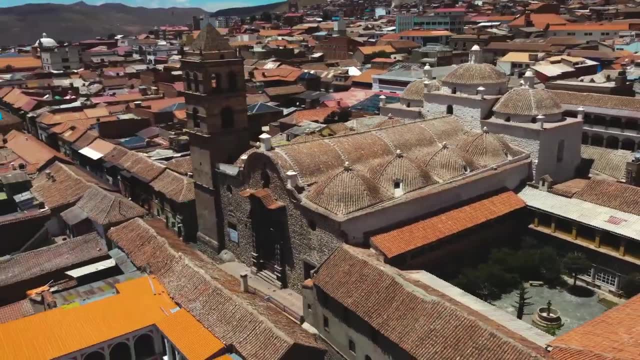 is because, in 1545, one of the richest silver veins in the world was found at Cerro Rico in Potosí, making the surrounding town one of the largest in the world, and its royal mint the financial institution that underwrote much of the world's wealth. 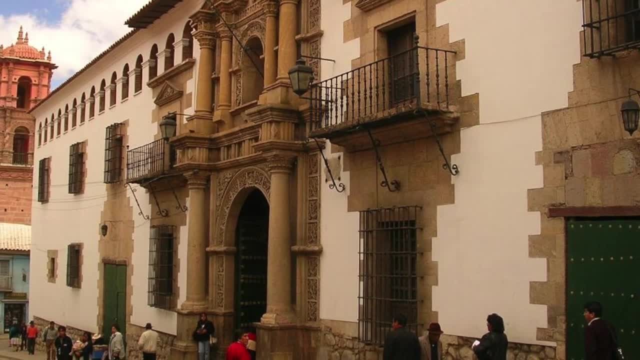 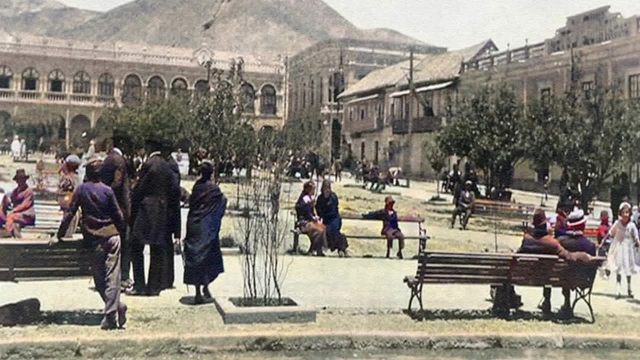 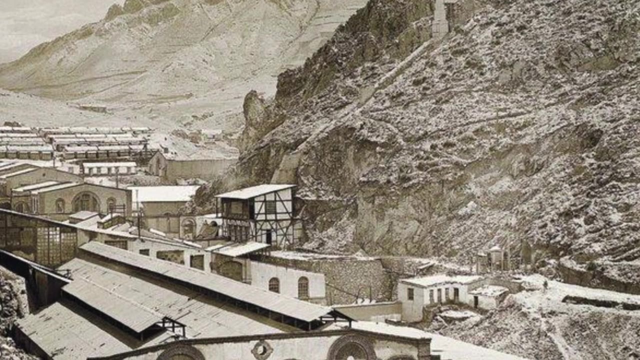 Potosí was not the only important mining center that developed. Nearby Oruro also produced silver, although its prominence came much later, with the production of tin, a commodity that came to dominate the Bolivian economy during much of the 20th century. 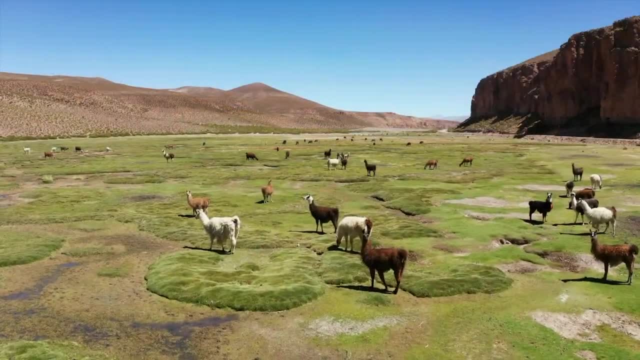 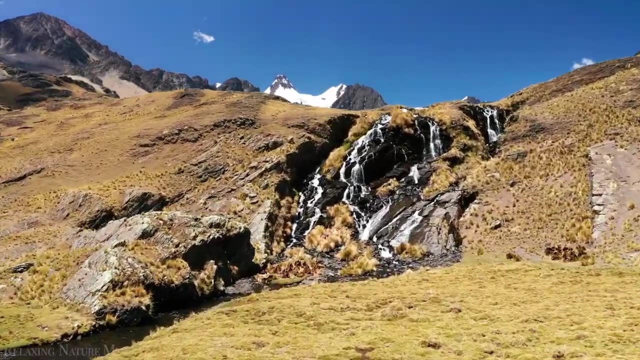 But not everything was a positive. While the altiplano produced much wealth, its mountain ranges also made political administration much more difficult, As geographically, it prevented communication and exacerbated political differences. One of these disagreements a dispute over whether Bolivia should be a centralized or federal system. 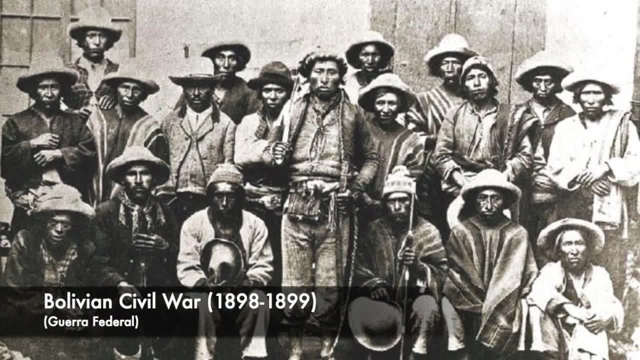 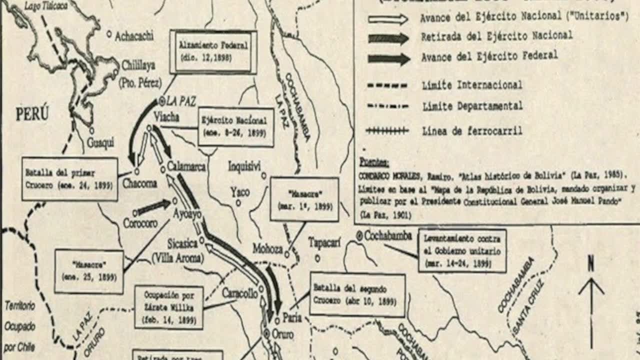 exploded into the largest civil war in the country's history in 1898.. The conflict was largely fought within the altiplano and it had the consequence of transferring the political capital from Sucre to La Paz, making the latter the seat of government with the highest elevation. 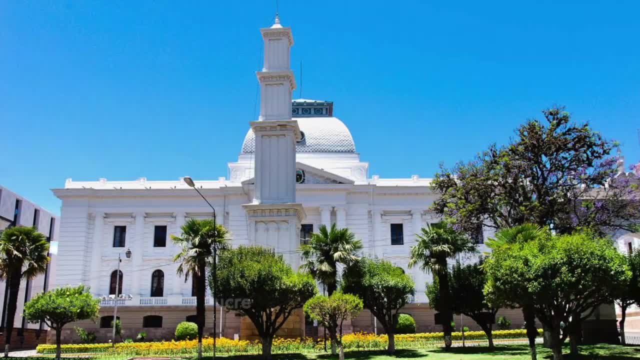 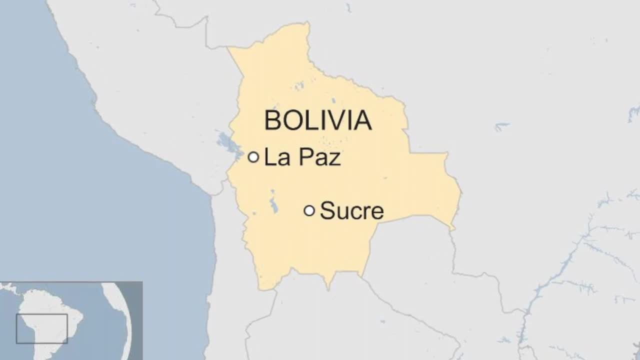 in the world. Although, as a compromise, the former retained the supreme court, This means that, technically, Bolivia has two capitals: Sucre and La Paz. Today, communications across the Andes are much easier, as modern highways connect the altiplano. 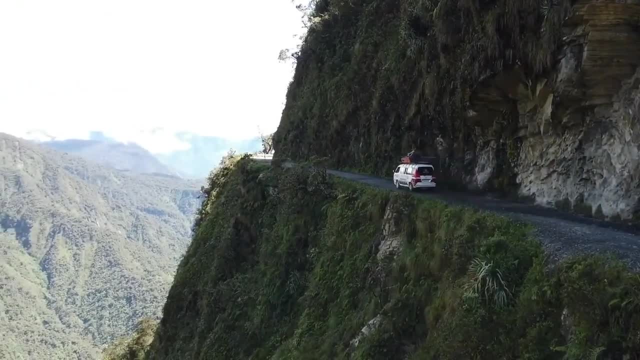 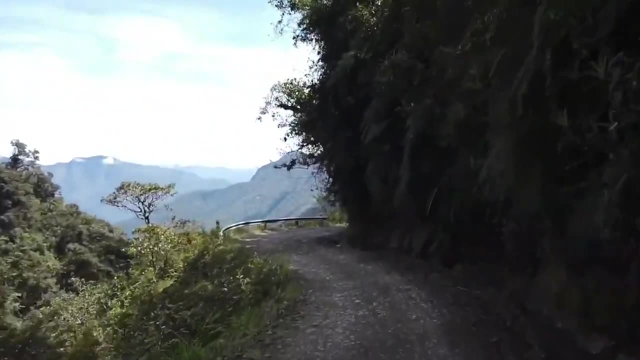 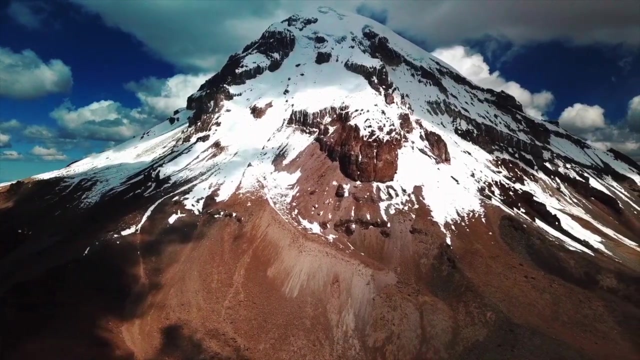 to the rest of the country, but it still retains the most dangerous road in the world, a stretch of about 36 kilometers or 20 miles, connecting La Paz to Coroico, where it is estimated 200 to 300 people die each year. The Bolivian altiplano features two other important sites. The first is 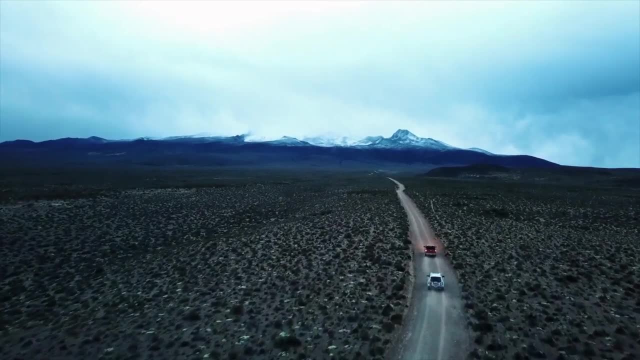 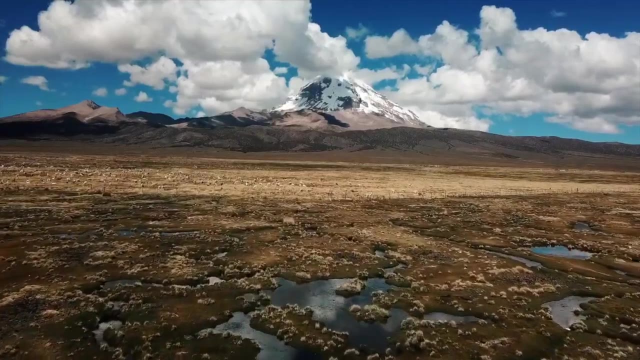 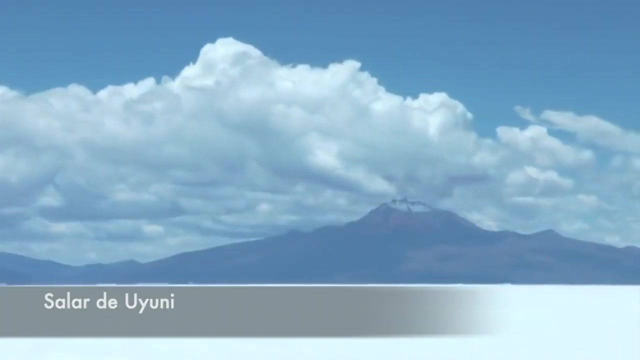 the oldest park in Bolivia and the ancient home of the Aymara people. It is an ecotourism hub because of its views and its flora and fauna, including endangered species like the Quirquincho or Andean hairy armadillo. The other is the Salar de Uyuni, the largest salt flats in the world. 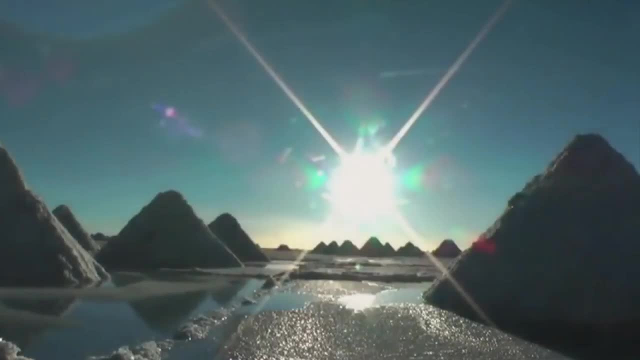 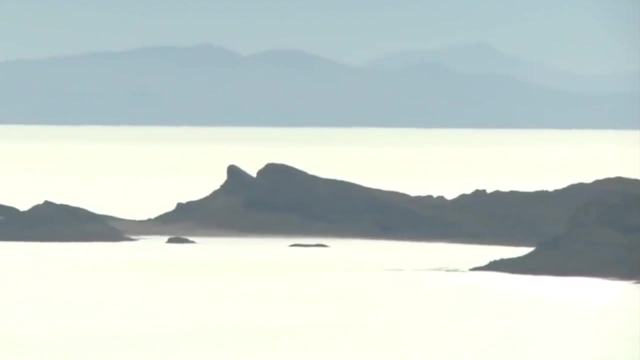 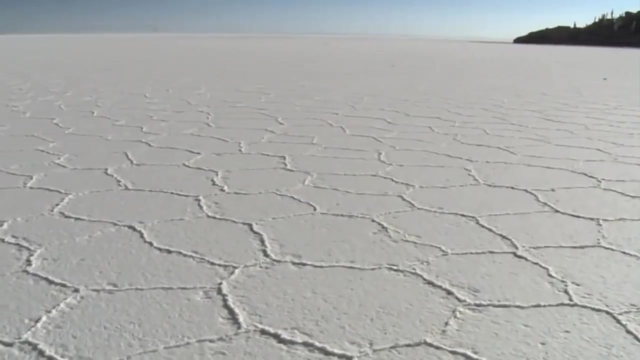 in a landscape that offers views like nowhere else on earth. Their impact in the economy used to be limited to tourists flocking to take pictures and film crews looking to shoot movies like The Last Man in the Sky, but the future seems to promise much more. That is because the flats are full of.